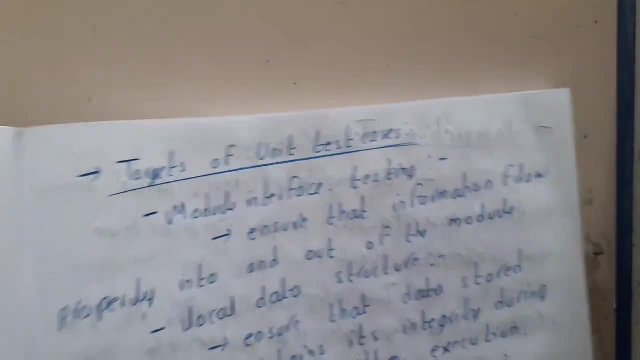 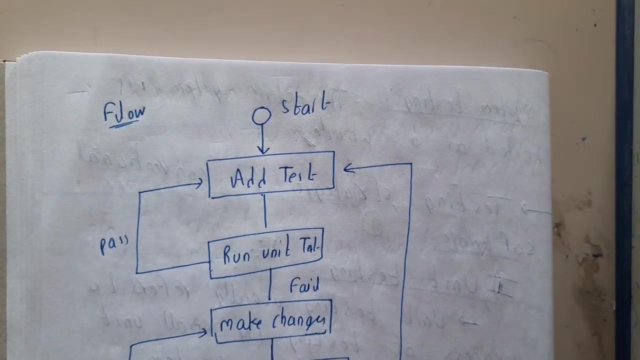 done again and again. so basically, you will be just removing the bugs, guys, to be clear, or errors, you can say: okay. so if you ask me to draw the flow chart for unit testing, it will be in this way, guys. so initially, before starting the unit testing itself, you will be writing the test cases, guys. 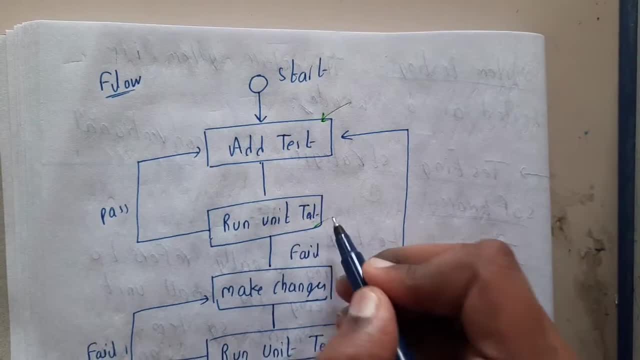 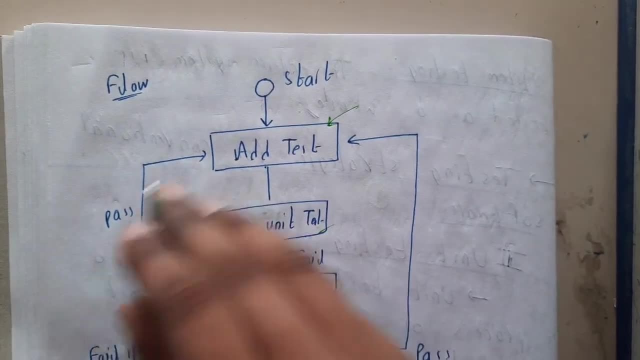 you will be adding some test cases. so then you will be running the test cases and if it fails, you will be making some changes. okay, if it passes, you will be adding one more test case and you again you'll be checking. this loop continues. if it fails, you will run the unit test. sorry, you'll make changes if it fails, you. 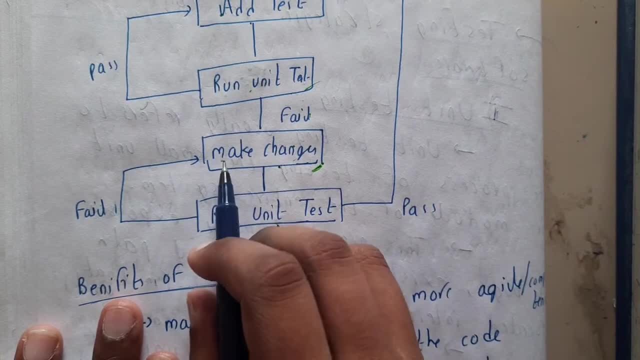 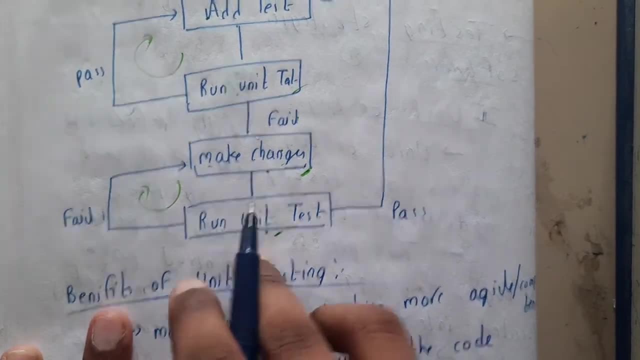 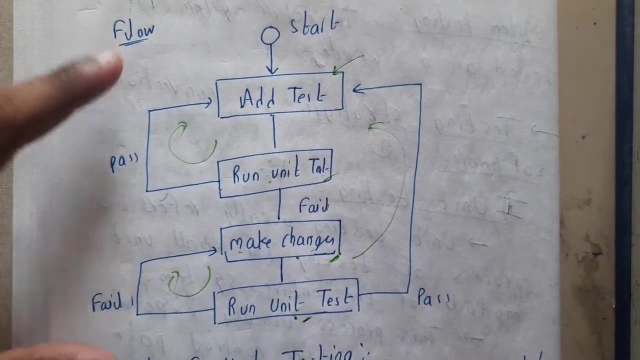 will make change and you'll test again. so if it again fails, you'll test, you'll make the change again. so, and this loop continues, okay, okay, if the- if this is true- it passes, it will come back and it will add new test cases and this group continues. so, basically, here we are, adding test cases, testing. 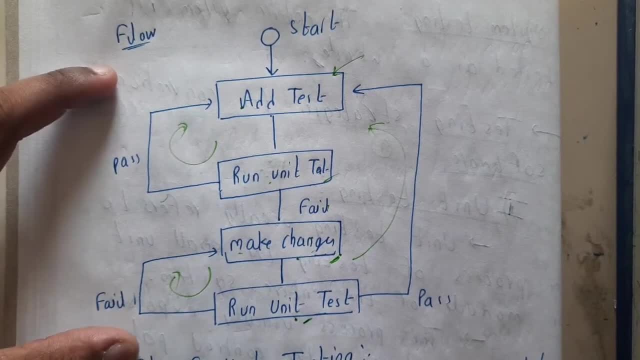 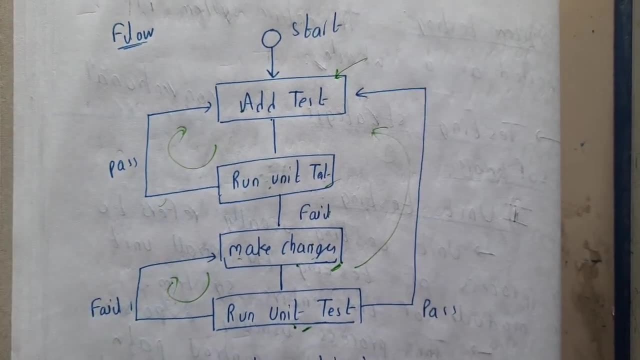 them if it passes the next test case. if it fails, you will be changing some things and you'll be retesting it. And if it again, if it giving some bugs, again you'll be retweaking it. So like that Okay. 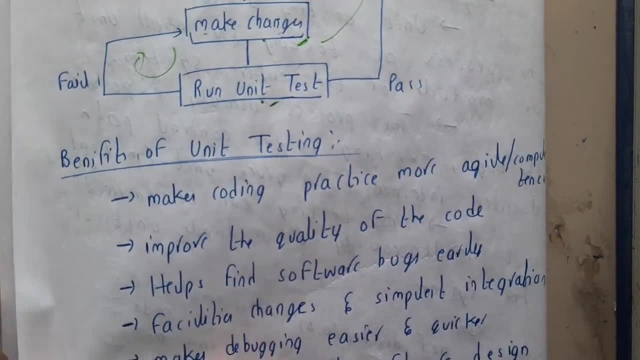 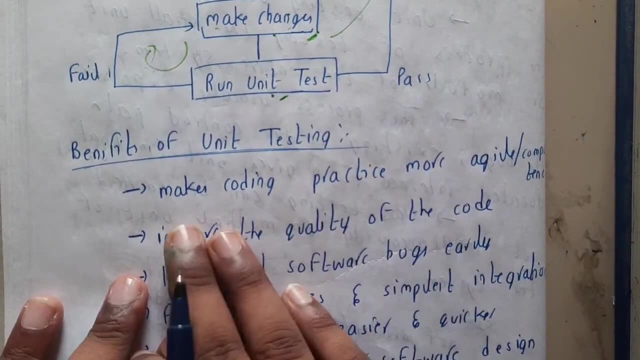 So you might be having a question that, okay, now we got some idea about unit testing, So are there any benefits or advantages? So there are many advantages, guys. It is removing your bugs right. So what else you want? So making code practice more agile and computer intense. 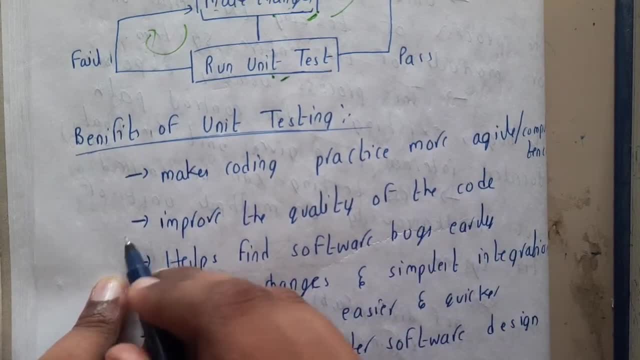 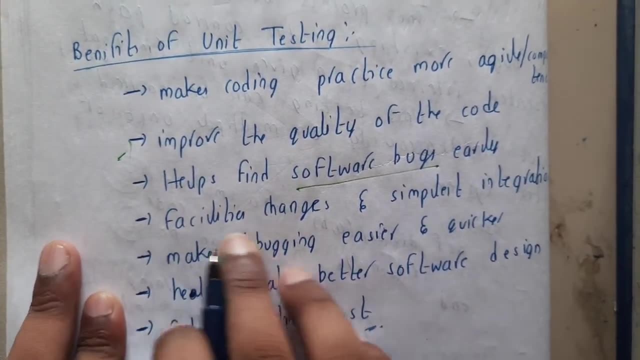 Okay. So more so improves the quality of the code. So basically, it improves the quality of the code, helps in finding software bugs earlier, early, early Okay. So facilitates the changes and simple integration. So integration will also be simple. 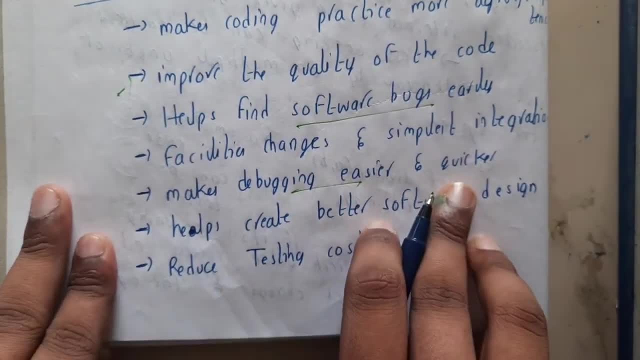 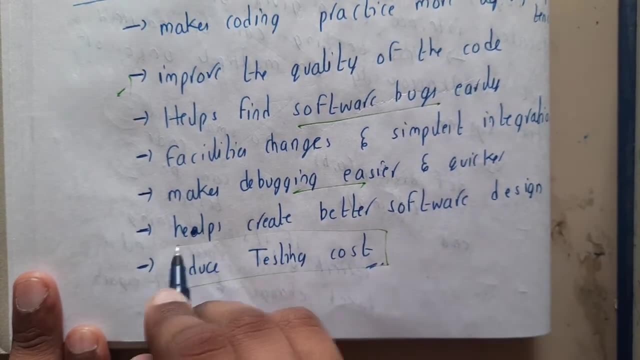 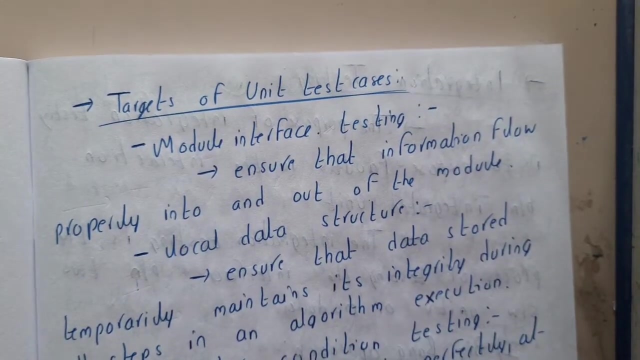 Okay Makes debugging easier and tweaks can be done quicker. Okay Helps in creating best software design and reduces the testing cost. So basically, unit testing is done when they are writing the code itself, Like when you write a particular module. you'll be testing in with some limited things. 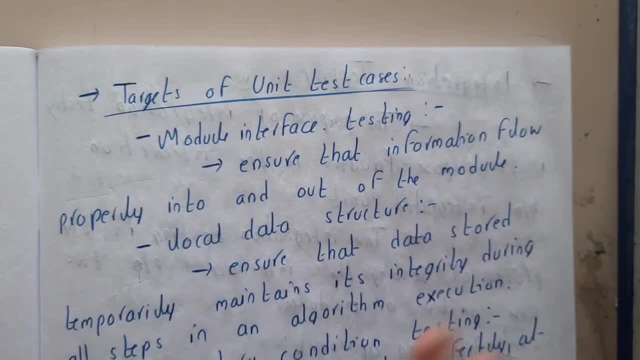 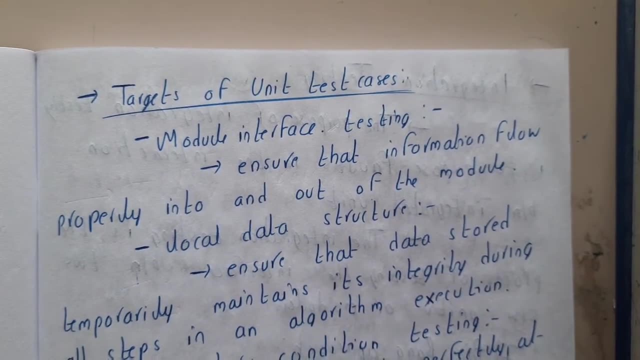 So that is also comes under unit test. Okay, So now let us go through. what are the targets of testing unit testing? So the top the points will might be repeating, as the benefits and the targets will be the same, right, Yes, 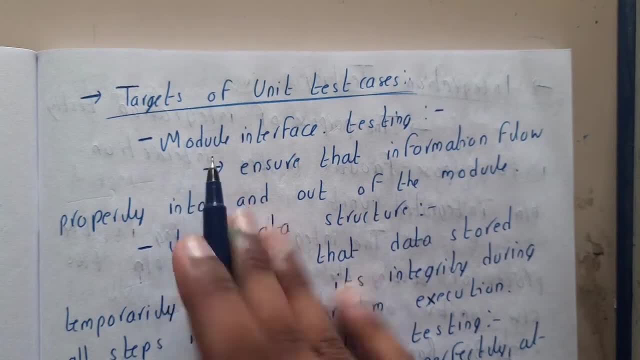 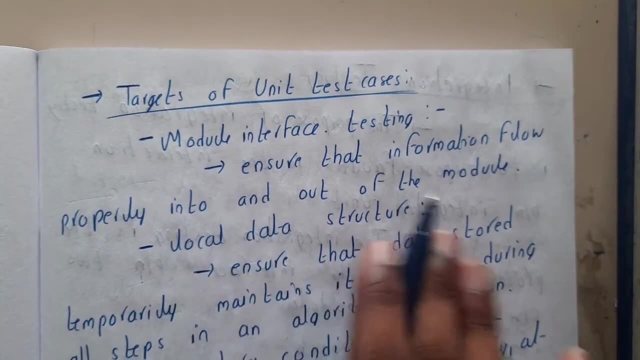 Module interface testing. So it ensures that module- I told you module is nothing but a smallest unit, So that we'll be testing it- So ensures that the information flow properly into and out of the module. So I told you what you'll be giving us: you'll be giving the input and you'll be expecting. 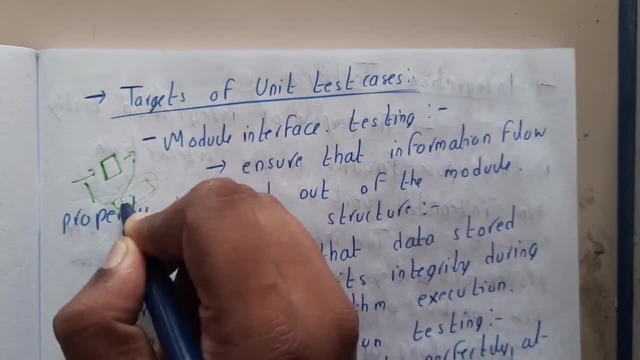 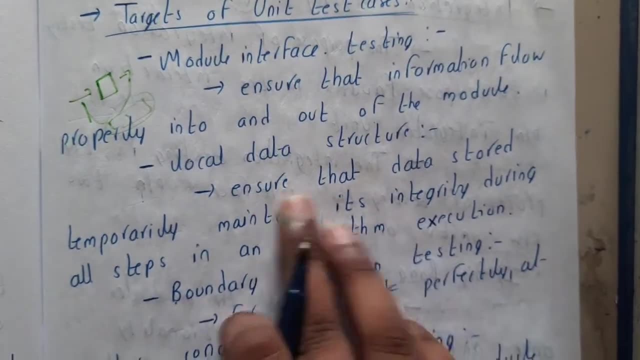 the output. So these inputs, So the input and output, should match according to your requirements, right? Yes, So that is what the testing will be done for. So local data structure. So ensures that data stored temporarily maintaining maintains it integrated during all the steps. 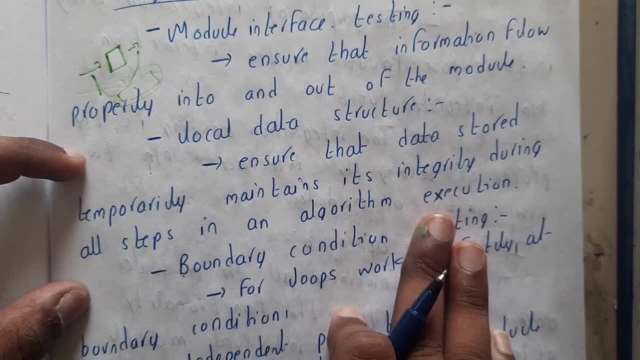 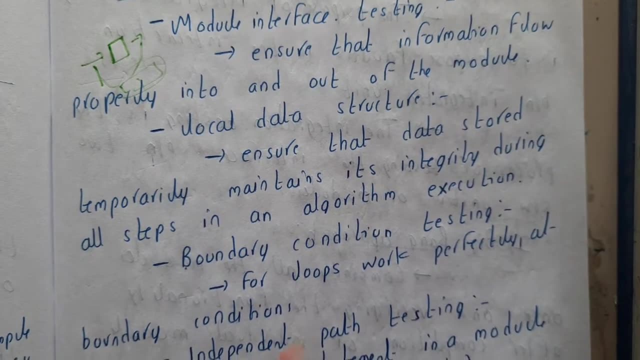 in the algorithm execution. Okay, So we will be checking, according to the local data structure, what data structure you are using. all the values are matching or not. Is there any tweaks in the structure? Is there any issues like that? So we'll be checking everything, guys. 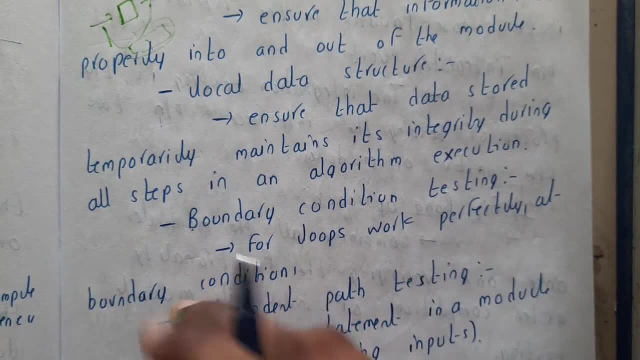 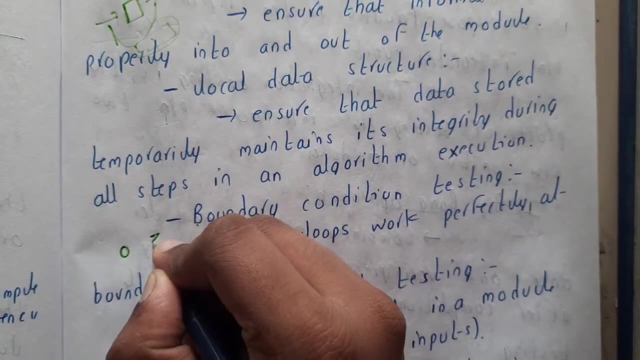 Okay, So boundary condition testing. So basically, So for loops. So whenever even I code, sometimes I'll be getting confused. So if I start from zero, should I continue till greater than or equal to 10, or only greater than 10, to print 10 numbers? 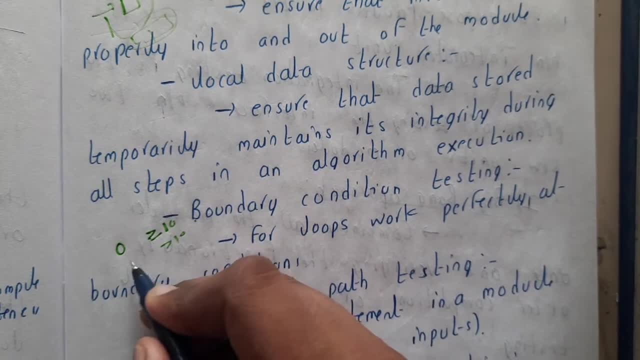 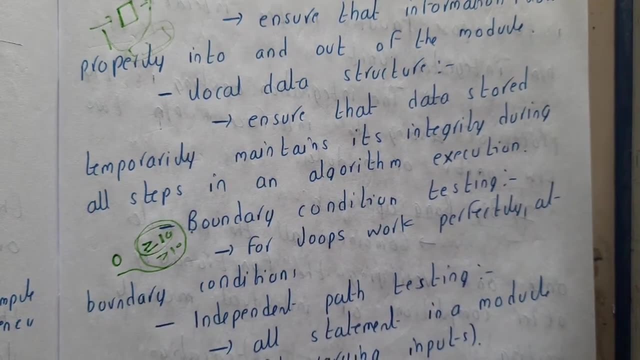 So most of us will be getting confused, right? Okay, So these are nothing but loop boundaries, guys. So at the end of where you are ending. So for these things you should manually check, like: once you greater than 10, after that you. 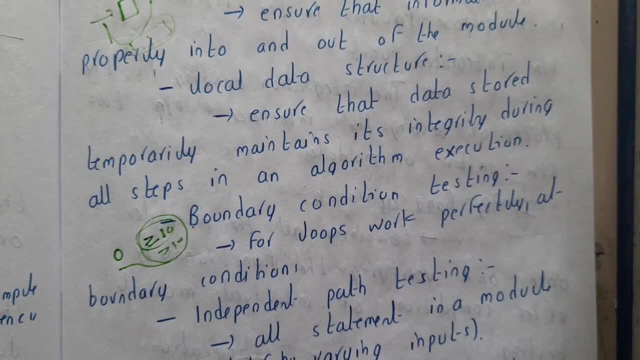 greater than or equal to 10, which is better performance or which is your requirement. So you'll be continuing with that. So in that way, you'll be testing it. You'll be testing those kinds of things. so independent path testing. 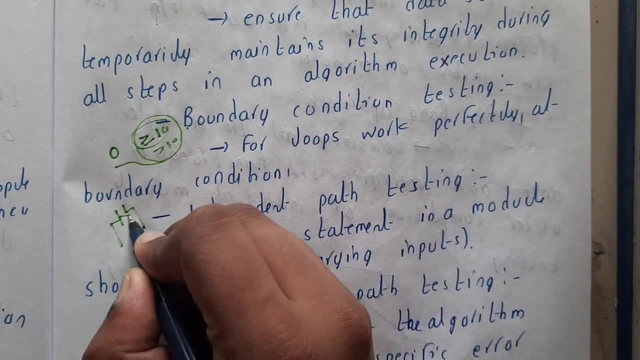 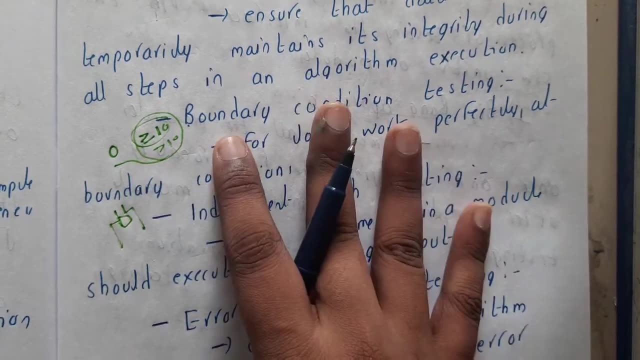 So basically, there will be multiple paths for a program. So whenever there is a particular decision, then there are multiple paths. with the single decision, we'll be getting two different paths. with the two decisions, We'll be getting four different paths. Guys will be discussing about these paths also. 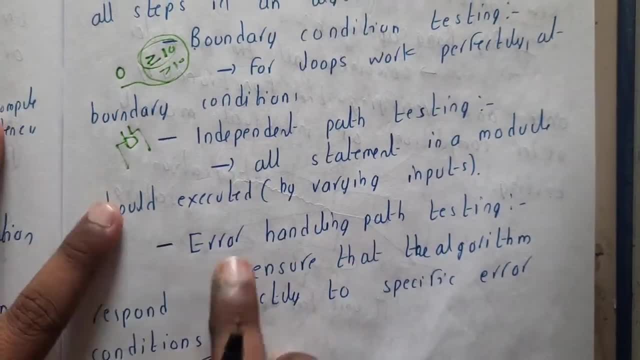 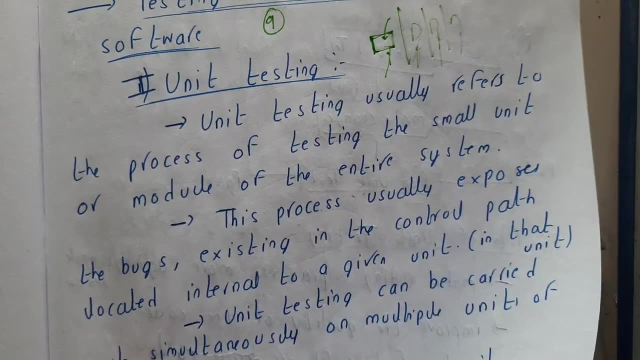 I think, in our future lectures. Okay So don't worry about that. Okay So, error handling: path testing. So, based on this path testing, you'll be handling the errors also. Okay So I hope everyone got some basic idea about unit testing, right. 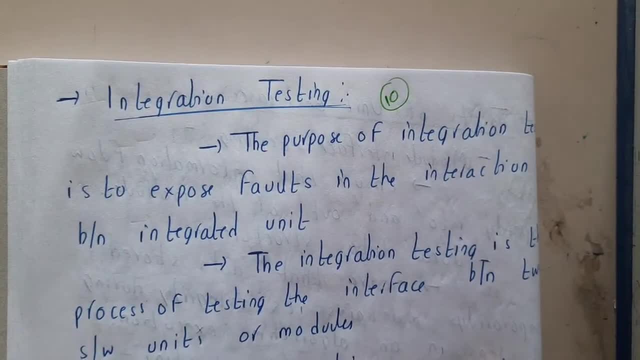 Okay, So in the next lecture we'll be going Okay, Through integration testing guys. Okay, So let us meet in the next lecture, Thank you. Thanks for watching.